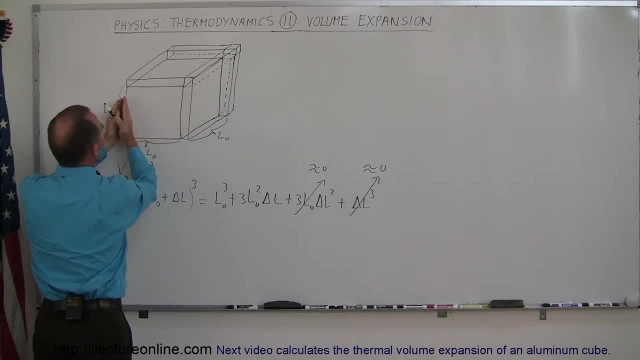 But imagine here that we have the original cube right here and it expands in this direction. so then, now that it's longer in this direction, it expands in this direction, so it's longer by delta L here. So let me show you this is my delta L here, over here, this is my delta L and, of course, in this direction, over here, this is my delta L. 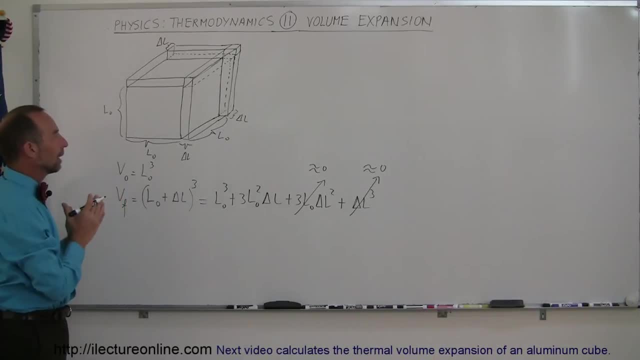 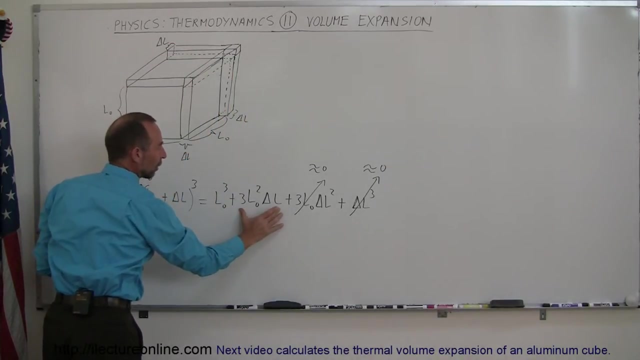 So you can see that in all three directions: length, width and height. this is my delta L. So we can now see that the three slabs- there's a slab on this side, there's a slab on that side and there's a slab on the back that's equal to this thing right here, that would be accounted for in this term: right here. 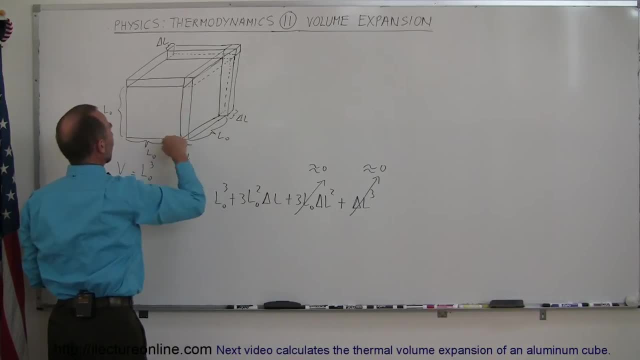 It's three times the original surface area of the cube, multiplied times a change in the length. Of course. when we do that, we get this slab volume like that. We have three pieces, and that's this right here Now. the next term right here is represented by these three little bars. there's a bar in this direction, there's a bar over here and there's a bar at the very end. that's, of course, also increase in volume. 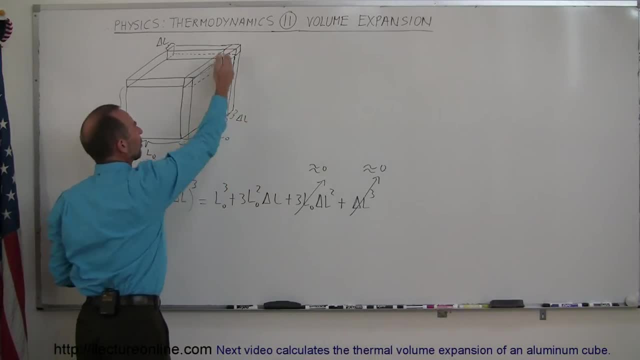 But those things are so small, since delta L is typically so small, that those bars- because it'll be delta L times the delta L times the initial length squared, and that's what we have right here, I'm sorry. no, delta L times delta L, so it's delta L squared times the original length. 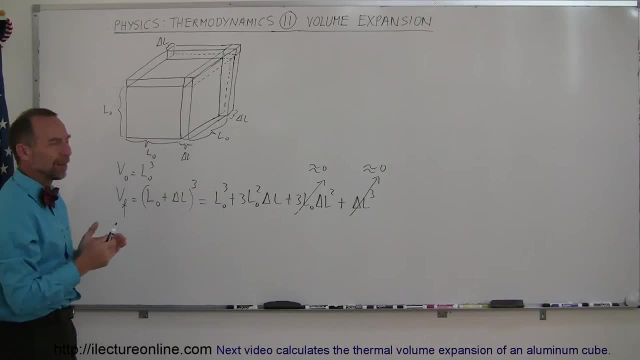 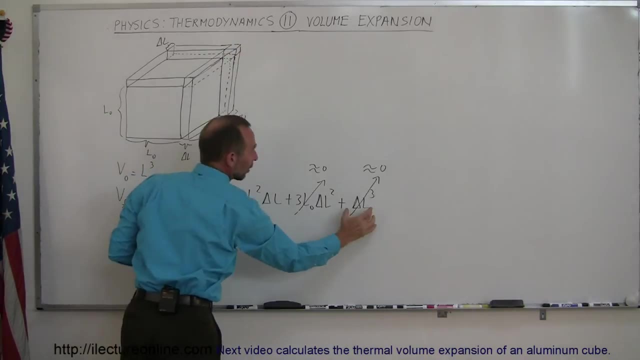 It is so small compared to the original volume that that's probably insignificant, And we can get rid of that as well. And then, finally, this little cube in the back which is delta L times delta L times delta L, which is represented by this term right there. that is so small we can ignore that as well. 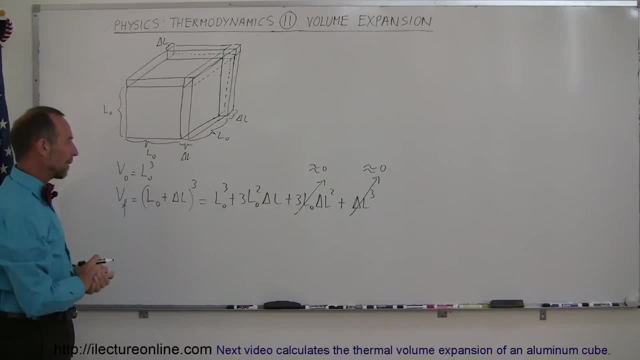 So let's, we'll see in a future example why we're able to do that. So if that's the case, we can go ahead and replace this by the original volume. so we can say: volume final is equal to the original volume plus three times L sub naught squared. times delta L squared. 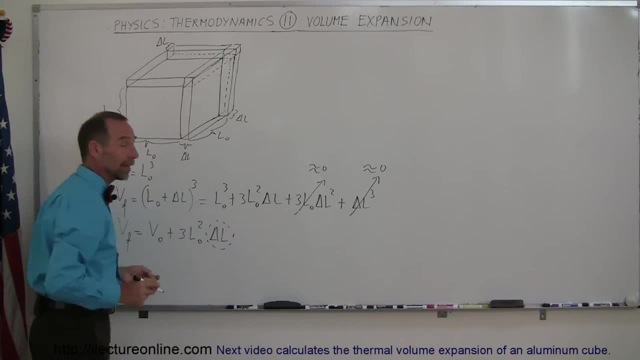 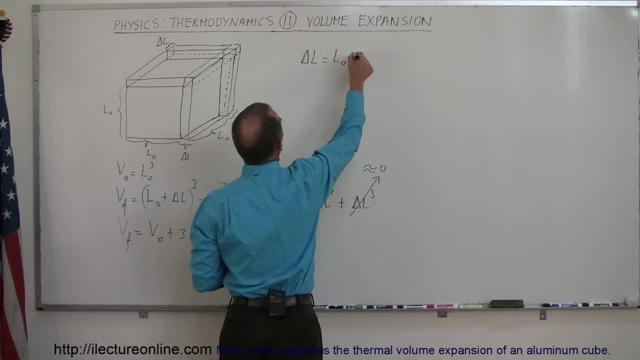 Now let's go ahead and look at this delta L right here and find the equation for delta L from our linear expansion And we can say that delta L is equal to L sub naught times the coefficient of linear expansion, times the change in the temperature. 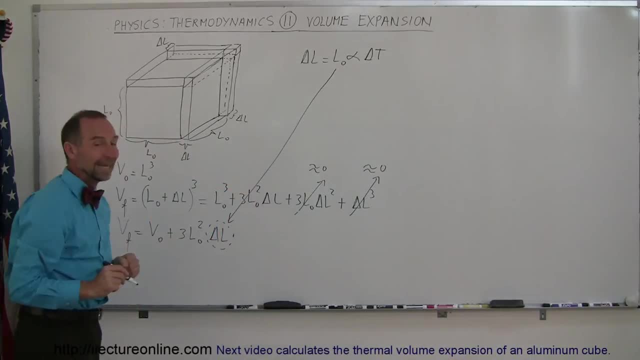 And take that and replace this in our equation. When we do that, we get the following: We get V. final is equal to V initial plus three L sub naught squared times this, which will be L sub naught times alpha times delta L squared. 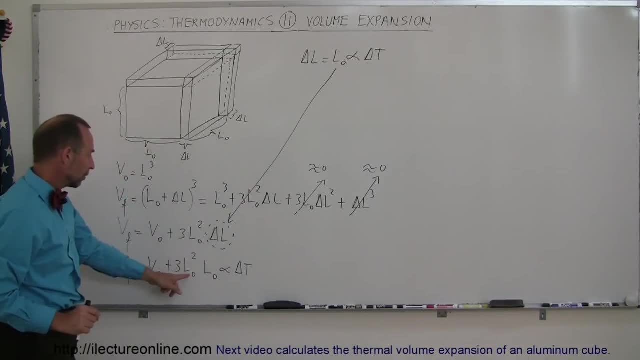 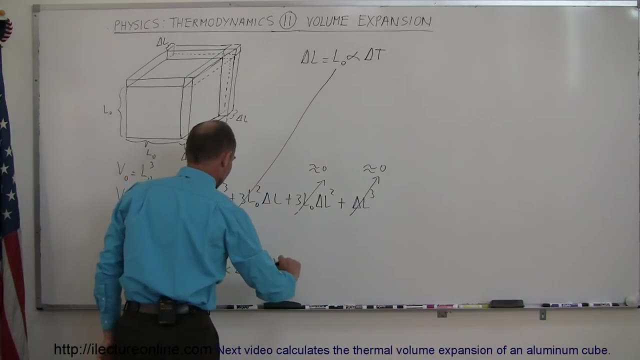 Now you can see that L sub naught squared times L sub naught is L sub naught cubed, And of course that's also equal to the original volume. so this can now be written as V initial plus three times V initial, alpha times, delta T. 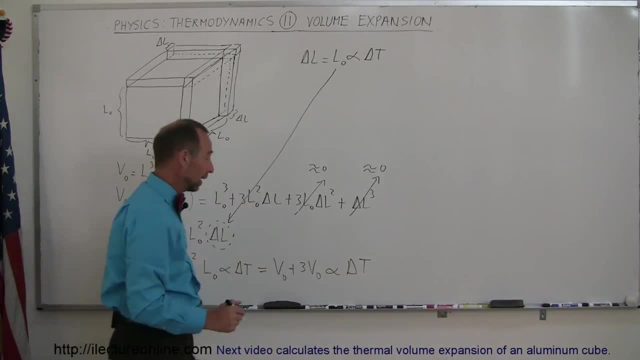 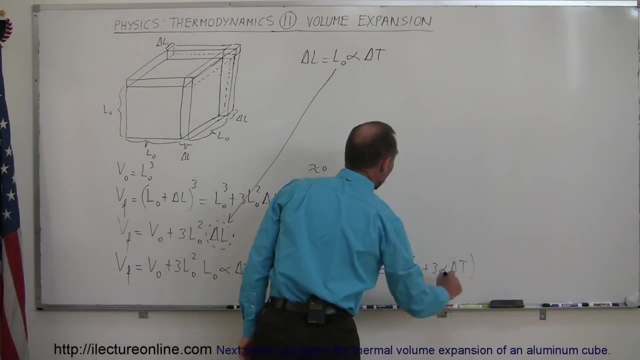 And then if you factor out a V initial from that equation, then this will be equal to V initial times one plus three alpha delta T. And then let's compare this equation to what we had when we did our linear expansion, Where L final is equal to L initial times one plus alpha delta T. 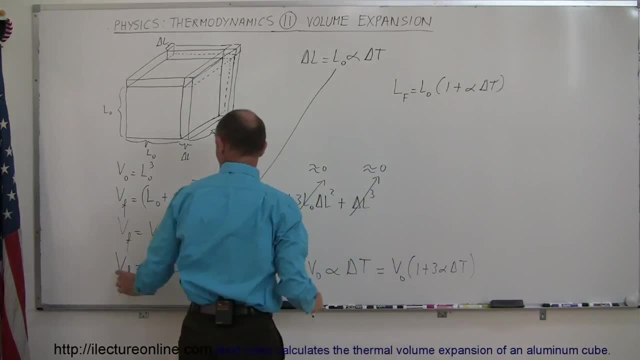 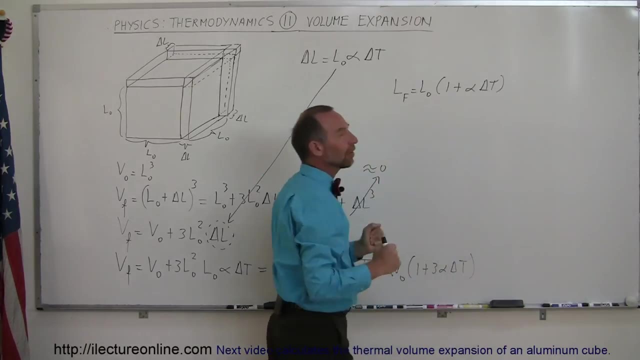 And notice the similarity between those two equations. Right here we have V final and L final. Here we have one plus three alpha delta T. There we have one plus one alpha delta T. And notice the only difference is the number three. right here. 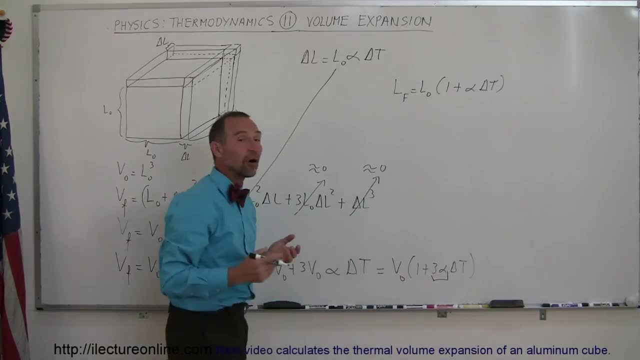 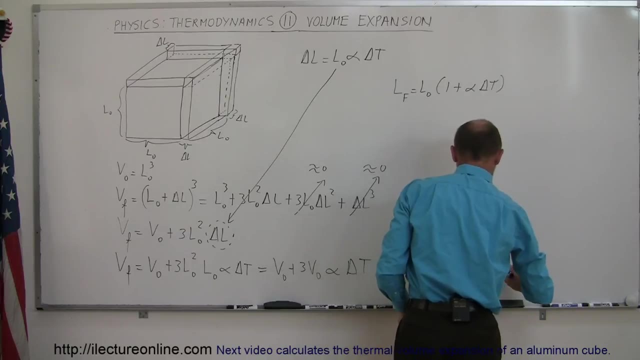 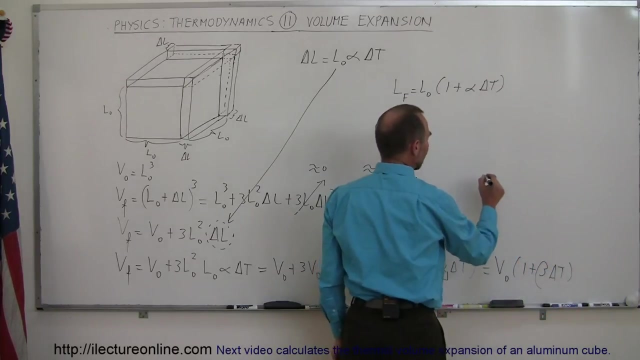 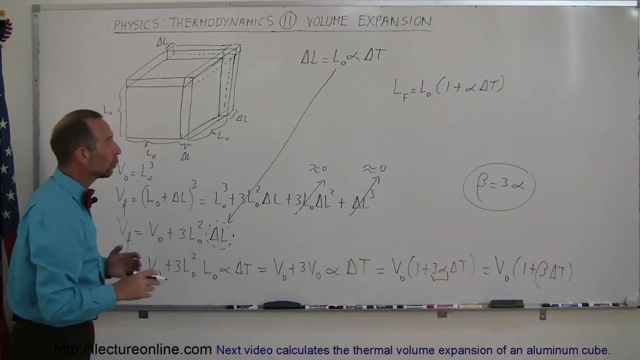 So this here is really the volume coefficient of expansion, And we typically use the variable beta, So this can be written as V initial times one plus beta times delta T. Understanding then that beta is equal to three times alpha. Now, when we're dealing with metals and wood and concrete and things like that, solids in general. 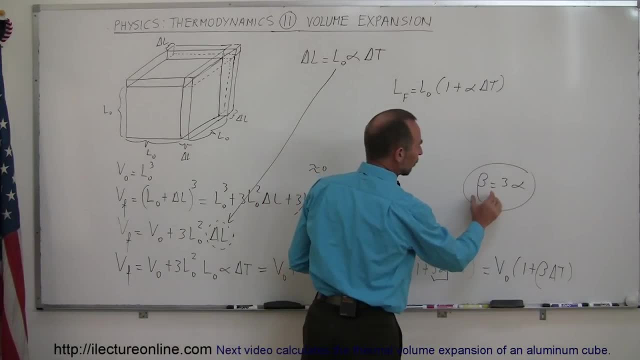 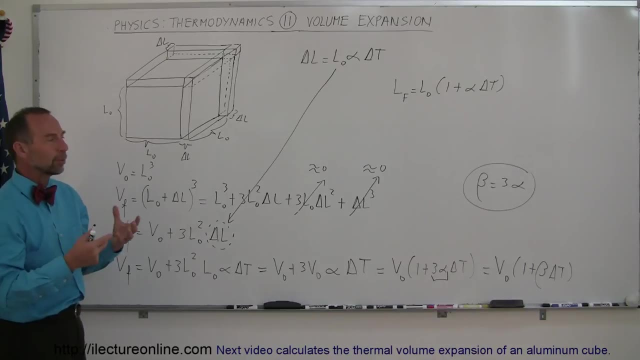 then we simply go ahead and call the coefficient of volume expansion three times the linear coefficient of expansion. But of course volume expansion can also be used for liquids, And so for liquids, typically in a textbook you'll see an expression for beta. 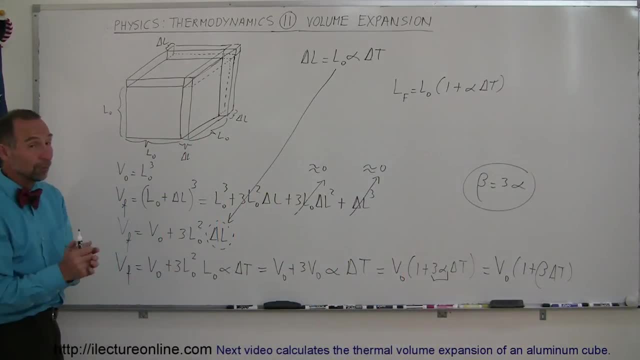 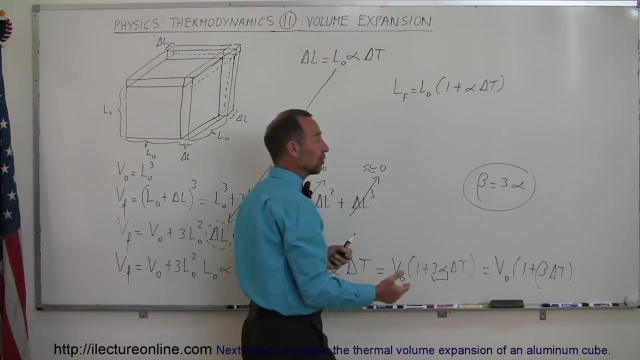 They'll give you the volume coefficient of expansion. Of course, don't multiply that times three, because then you'll get the wrong answer. So if you're given the volume coefficient of expansion, use it. If you're given the linear coefficient of expansion, make sure you multiply that number by three.